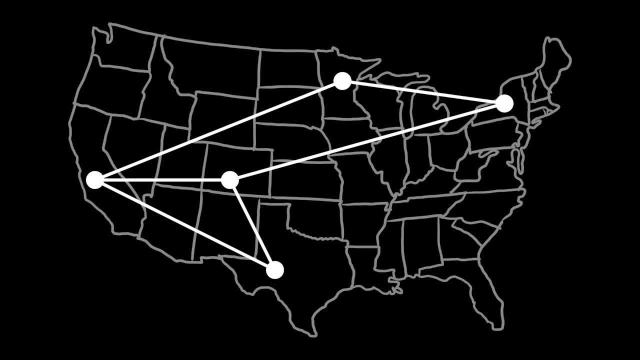 to New York, and then to New York, and then to New York, Minnesota to New York, then we would have something to work with. At this point. the map in the background is no longer useful If we already know that these are the three cheapest options. 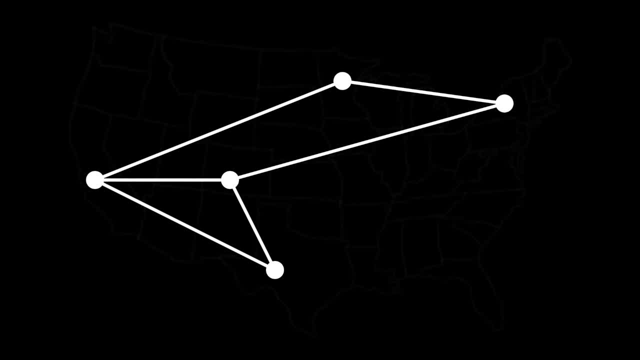 then these are going to be the only ones to consider. Suppose the prices of the flights are as follows: Now it's easy to see that the flight through Minnesota would cost $300 in total, the flight through just Colorado would cost also $300 in total, and the last 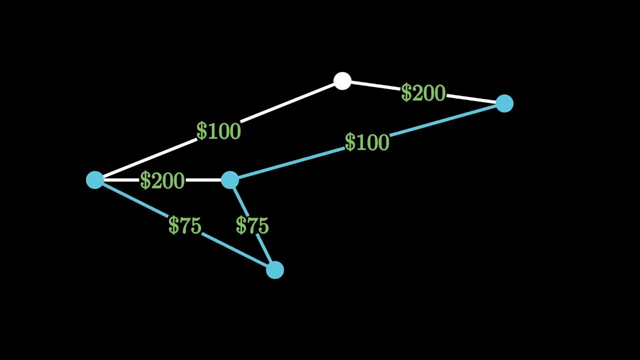 flight going through Texas, then through Colorado would, of course, cost only $250.. So, even though we have to go through Texas and Colorado, this does end up being the cheapest flight. In a more abstract sense, what we wanted to find was the path which is connecting California. 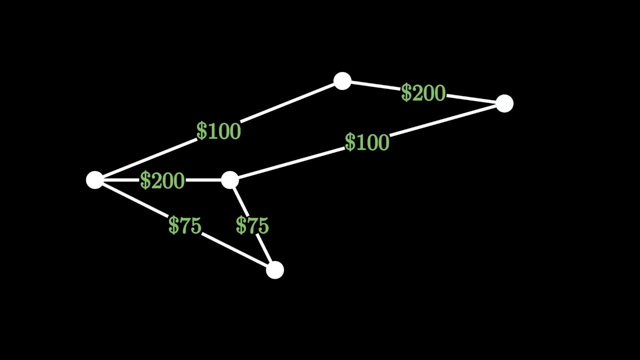 to New York but also collectively has the smallest weight In this graph. it wasn't really too difficult to find this path, but you can imagine that there are typically more than 3 flights going from California to New York, And to tell a computer to find the path of. 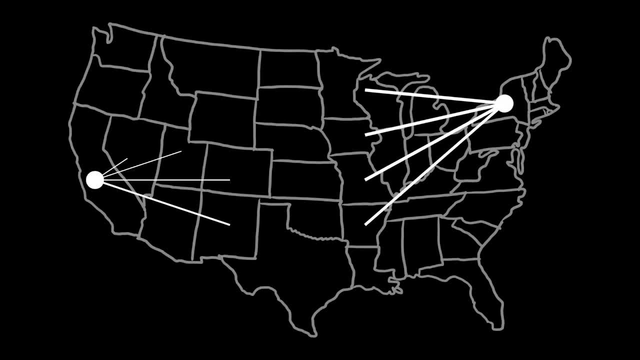 the total smallest weight. going from California to New York is a pretty difficult task if you're considering every airport in the United States. Additionally, we would have no clue what that graph is going to look like. This is just one example where you'd want to study. 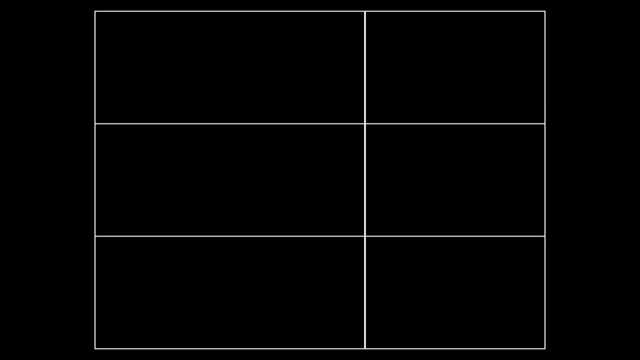 a graph in the abstract. Some people will start this journey by looking at a couple of different graphs. First, the most common is to look at the complete graph. This is the graph which contains every possible edge. We could also look at a cycle graph, or even maybe a path graph, But whichever graphs you choose to study, 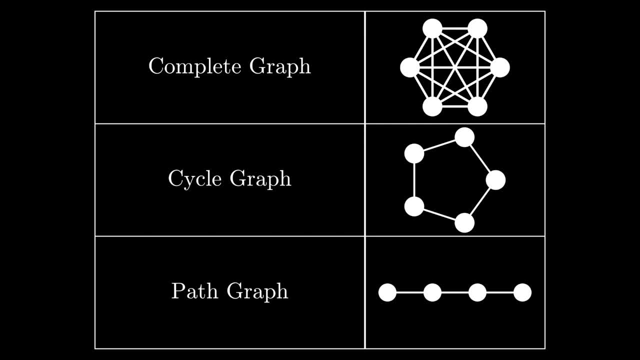 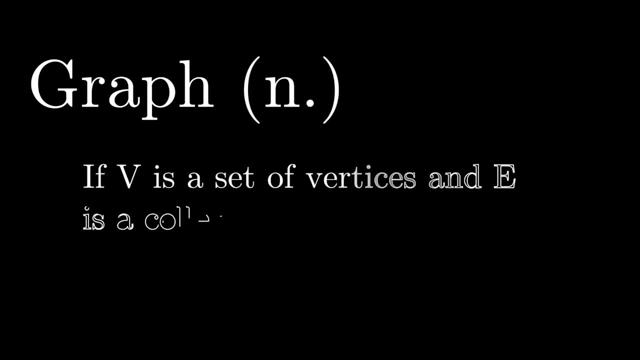 it's probably good to know what the abstract definition of a graph is. We say that if V is a set of vertices and E is a collection of vertex pairs, then the tuple ve together is a graph. The next most helpful video that I, when I have my computer on it, is the one about checking. 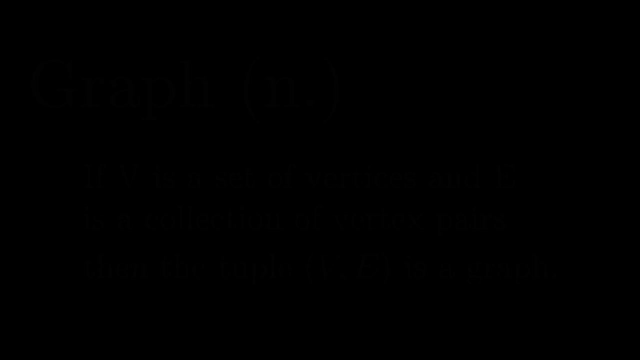 the exact coordinates of the top of the plane in order to find the path. The graph in this recommend would be on the adjacency matrix or the incidence matrix. These two matrices are normally how we tell a computer which graph we're talking about. Of course, this isn't the only way to continue, but whatever you choose to do, I 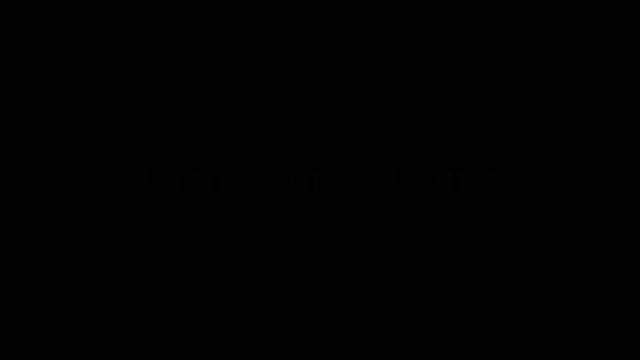 wish the best of luck to you and I hope you join me again soon.